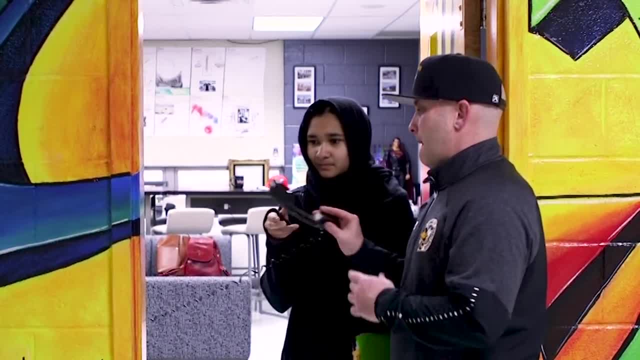 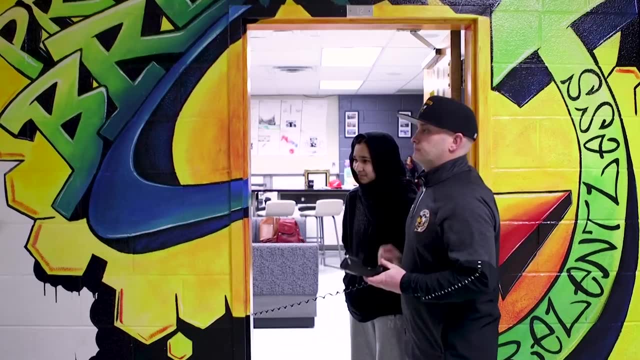 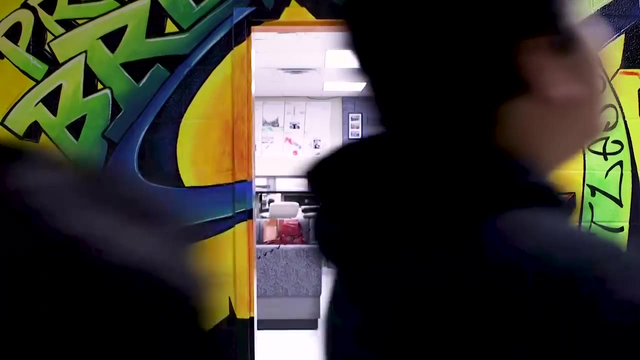 that were lost in that tragedy. A minute of silence begins now. Hey, great job, I'm proud of you, Love you All right, terrific job. Remember, put your cell phones in your lockers. Remember, take care of your business. today I've been at Fred Lynn a year and a half and 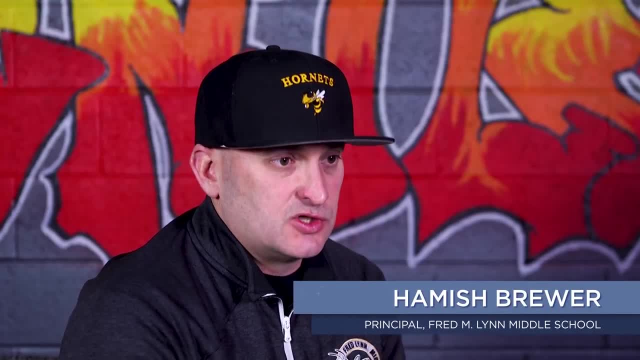 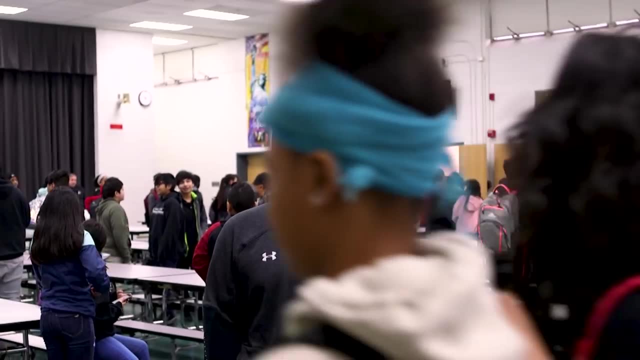 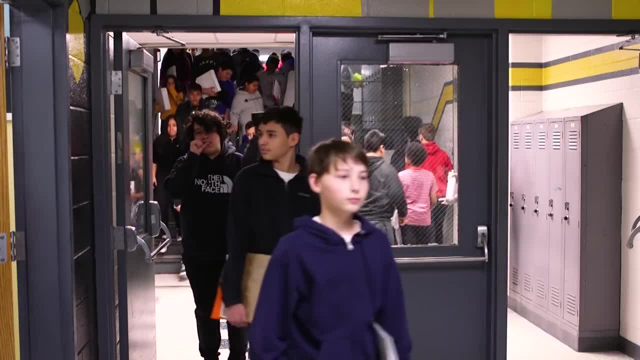 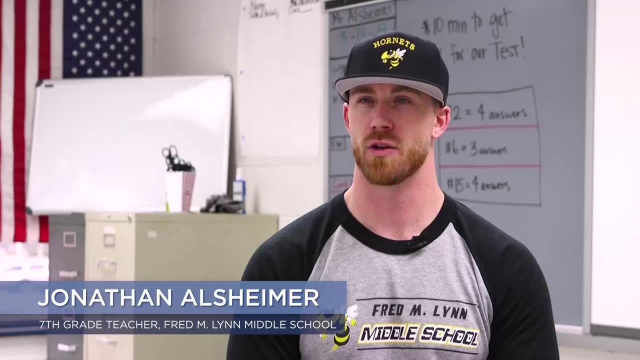 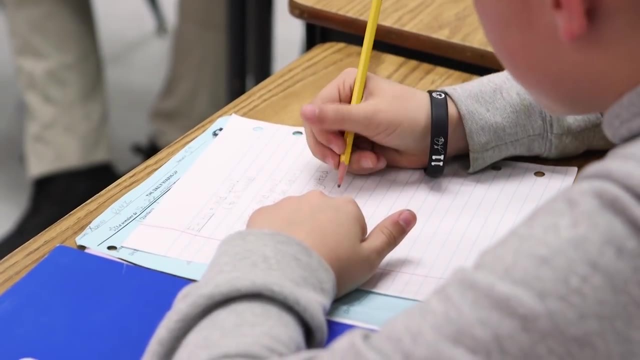 We've managed to turn this around in a year and a half. In the beginning, people were so frustrated with the way things were going that there really wasn't a lot of student-centered learning. You know, I think most people were just trying to keep their head above water with giving worksheets, reading out of the book and that. 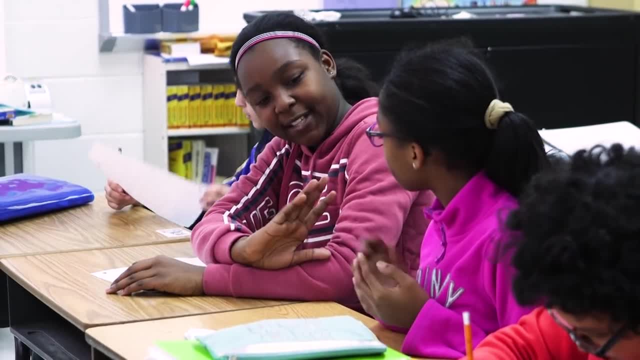 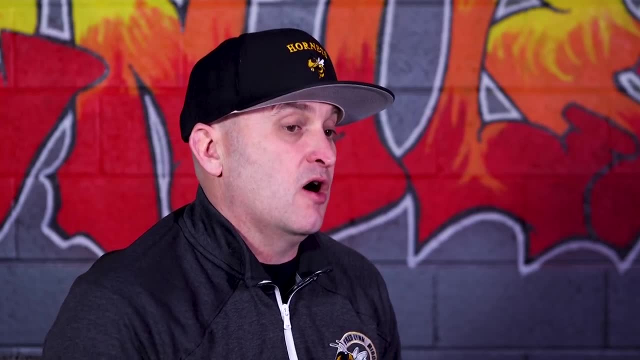 was pretty much all you saw. We've made a number of changes in our building. To be strategic, we've made a number of changes in our building. One of the things that I've done everywhere I've gone is I've moved my office to the middle. 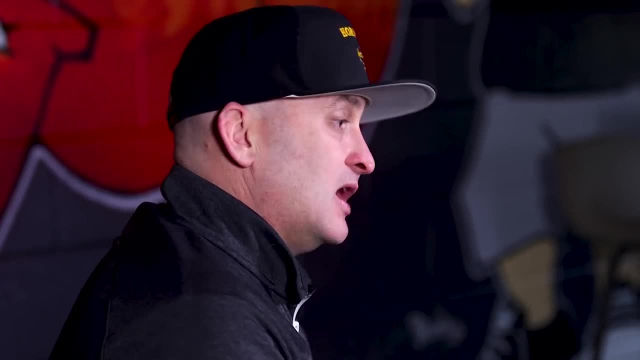 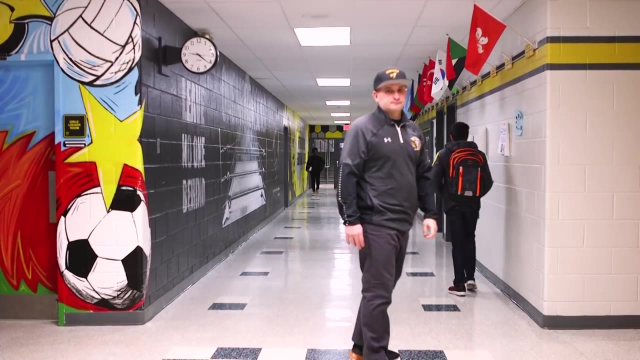 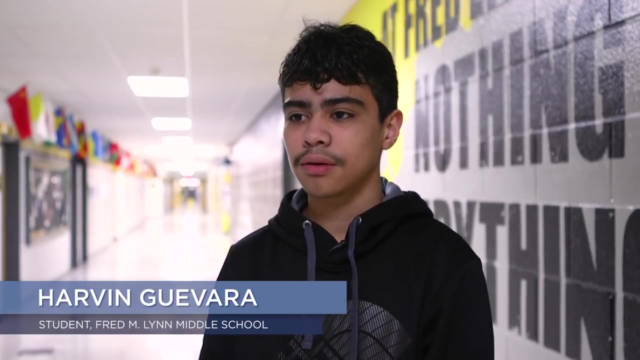 of the school. My job is to be in front of my kids, available for my kids, ready for my kids, helping my kids and serving my kids. When I came to the school in sixth grade, the building looked ugly, All white, yellow colors and that's it. Then Mr Brewer came and he changed the whole look. 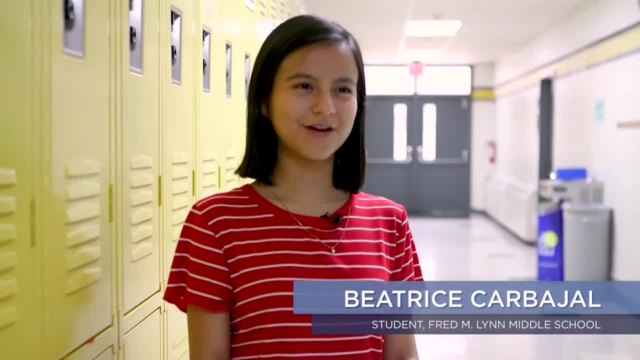 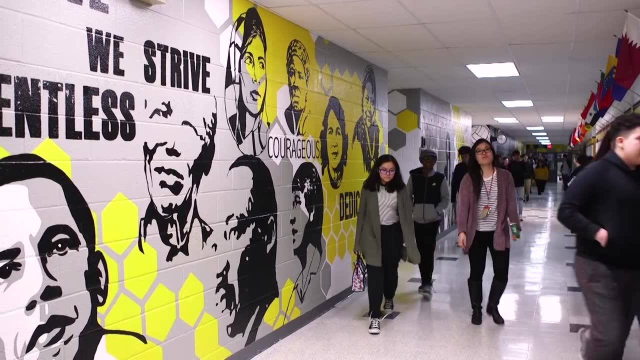 of the school. He has a lot of motivation stuff. He took down this mural, he put motivation pictures and who inspired us? The murals go beyond just being a cosmetic upgrade to a building. Your building becomes the expectation you set for it. 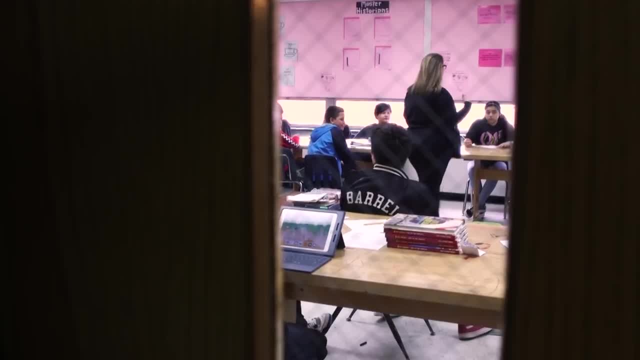 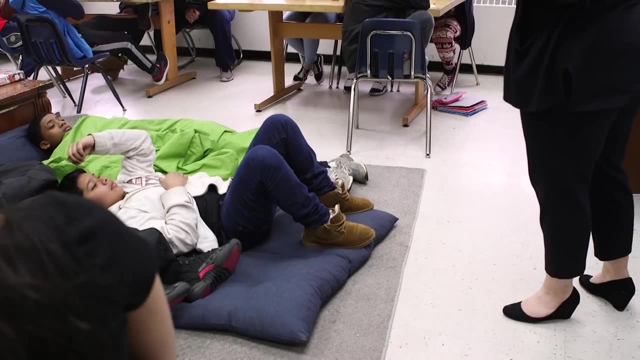 I want you to look at the number line on the bottom. Okay, I am a big proponent of flexible seating. I love the idea of a kid being able to come in and pick where they sit, and pick how they learn. It's about the kids. It's what's best for the kids. It's not necessarily what's easy. 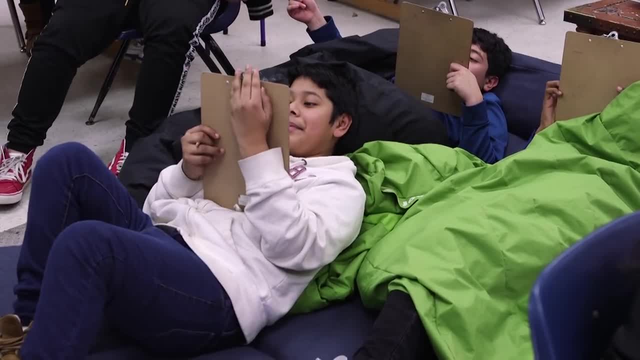 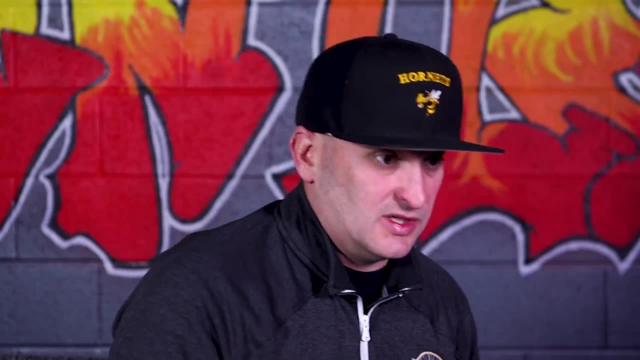 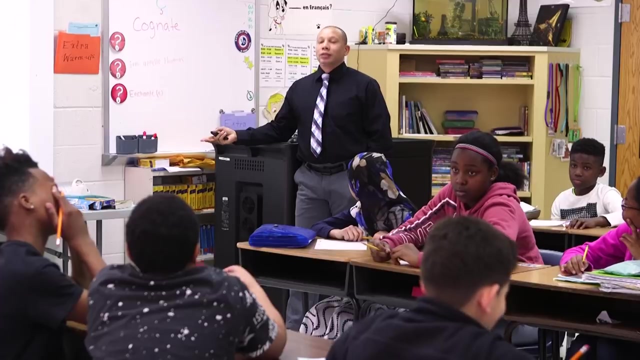 for me or what's best for me. When kids feel loved and respected, they're willing to take more risks, And that's what I'm seeing. Our participation in the classroom is up because they're excited to come to school and participate in the learning process, which means student discipline has come way down because kids